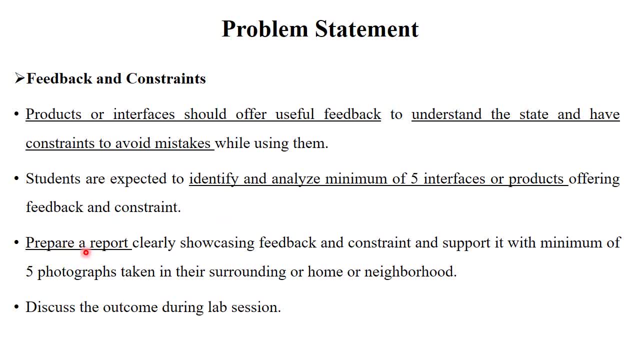 or products offering feedback and constraints. You need to prepare a report clearly showcasing feedback and constraints and support it with minimum of 5 photographs taken in their surrounding or home or in neighborhood, and discuss the outcome during the lab session. So this is the problem statement mentioned in your syllabus. So let's see the first. 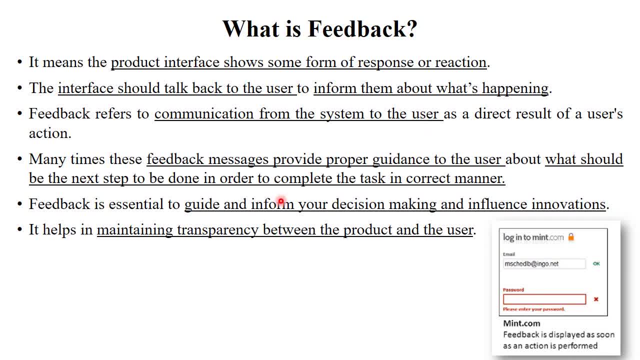 First we will understand what exactly feedback and what exactly constraints. So first, what exactly feedback? So basically, feedback means the communication between the system and the user, Whatever the appliances we use- we use refrigerator, washing machine, then TV, mobile. 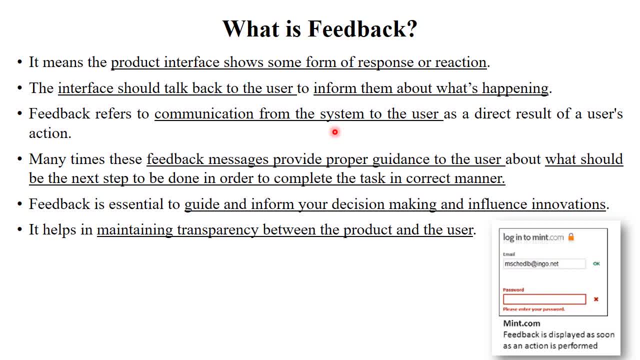 laptop. So each and every communication between the system and user Means system give a particular notification, particular message and user need to follow those message. This concept is called as feedback. So basically every product interface having a particular response or reaction message is there right So many times. this feedback message provide a proper. 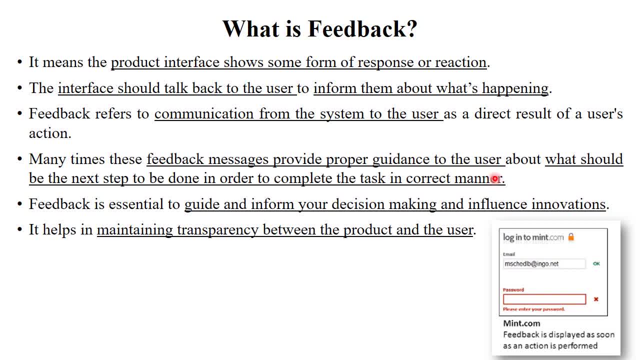 guidelines to the user Means how to use a particular application and what should be the next step in order to complete a particular task in correct manner. right, So this is called as feedback. So, basically, feedback is a guide and inform your decision making. 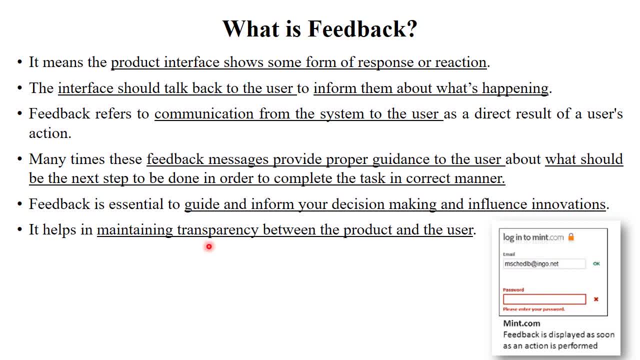 and influence innovation. Basically, it helps to maintain the transparency between the product and the user. Just take one example here. Suppose any login system. You need to login a particular system by using email or password right, And when you enter an email and your password box is incomplete. 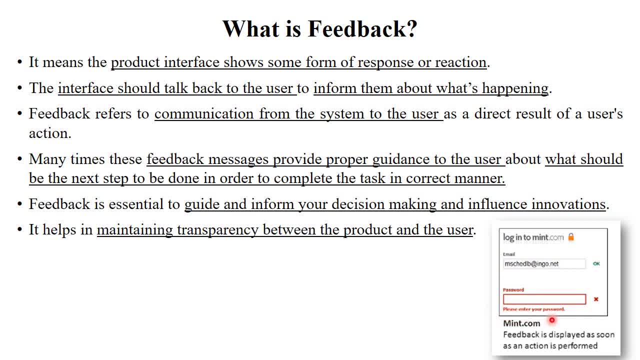 or empty. So at that time they give a feedback like: please enter your password, Otherwise you don't move to next slide, right? So this is called as feedback. So basically feedback means message that provided by the system to the user. 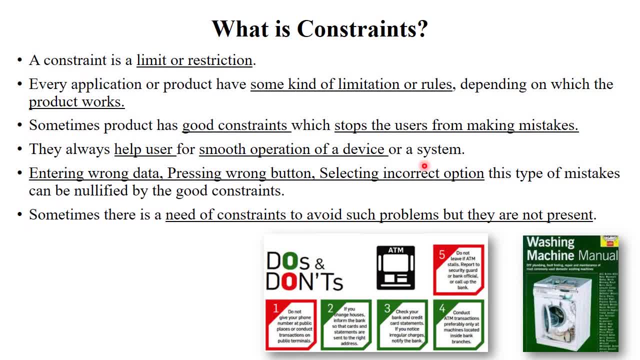 Correct Next. Now, the next point is: what exactly constraints? So basically, constraints means limits or restrictions, Every application or every product having a particular kind of rules or limitations. right See, when you purchase a particular application, like suppose you purchase refrigerator, or suppose you purchase TV, So at that time there will be a particular 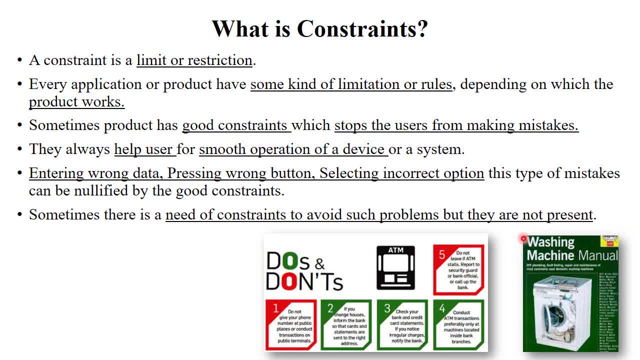 lab manual. right, Like when you purchase a washing machine, so there is a manual. is given that particular manual, each and everything have mentioned how to use do and don't regarding washing machine right. So this manual is called as constraints means they provide a. 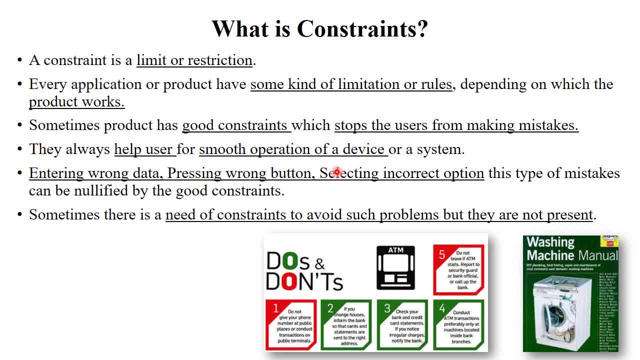 particular limitations, particular rules, particular restrictions on the particular using of that particular application right. So if there are good constraints, so you need to follow those constraints because they stop the user from making a mistakes. You need to follow that rules. 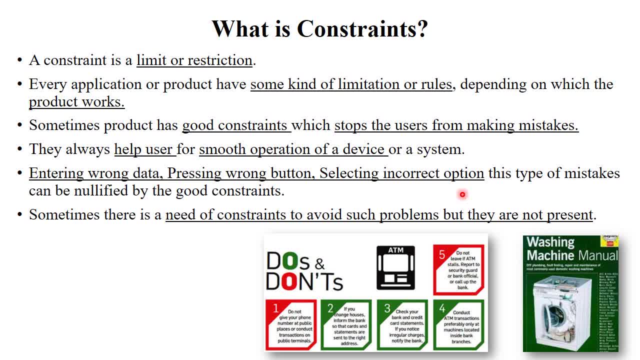 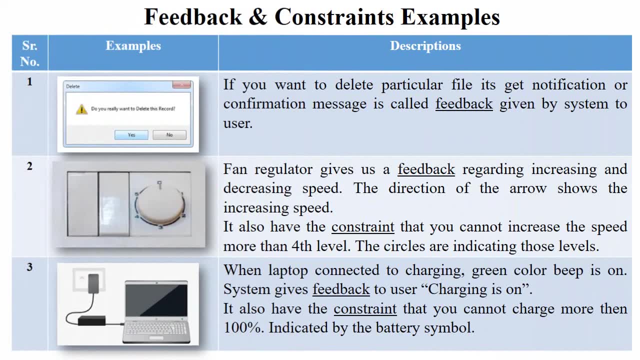 If you can entering a wrong data, Pressing wrong button or selecting incorrect option. These types of mistakes can be avoided by using the constraints. That's why every user you need to follow those constraints before using any applications. Next, Now see here. These are the some examples related. 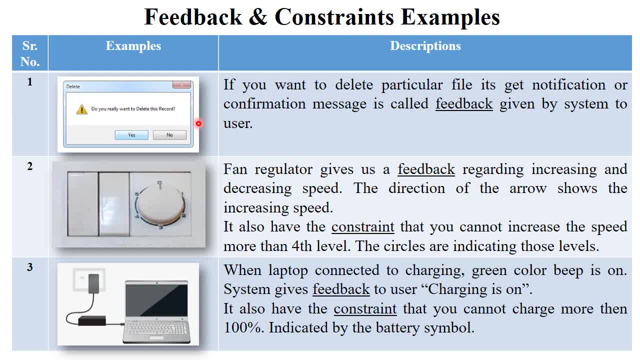 to the feedback and constraints. So you need to mention these examples in your assignment and make a proper report of this particular examples right Now. the first example is right. So when you want to delete a particular file or particular folder, your system give. 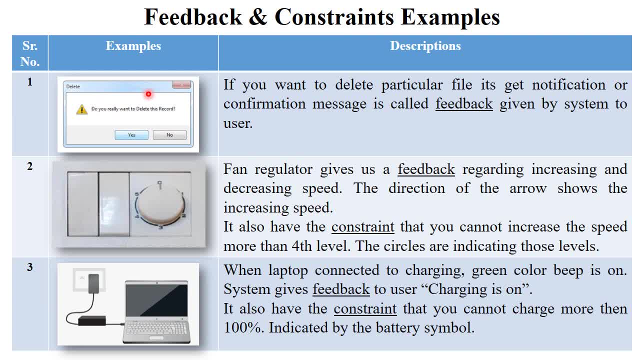 you the message: Do you really want to delete this record? right, So this is called as feedback. or this is called as confirmation message. right After that you need to press yes or no, So this is called as feedback. Next one is see here: fan regulator in your 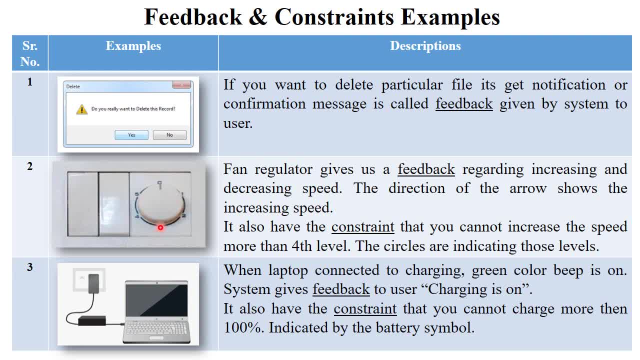 fan regulator. A particular feedback is given by using this refrigerator, by using this regulator button. Okay, see here This regulator button. You can see that this regulator button is used for increasing and decreasing the speed. right This arrow arrow indicate the 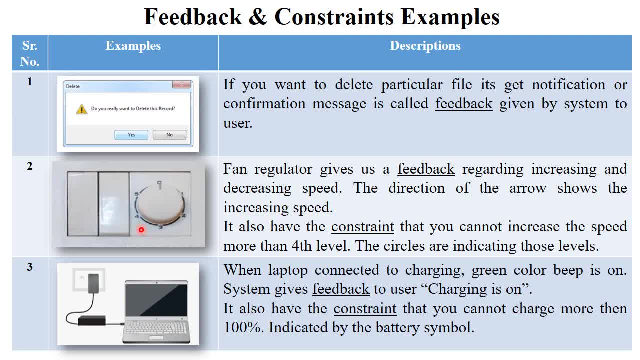 increasing speed. So this is called as feedback, and constraint is you can increase the speed up to the fifth level right, Like 0,, 1,, 2,, 3,, 4 and 5. Not more than that- 5. This is called. 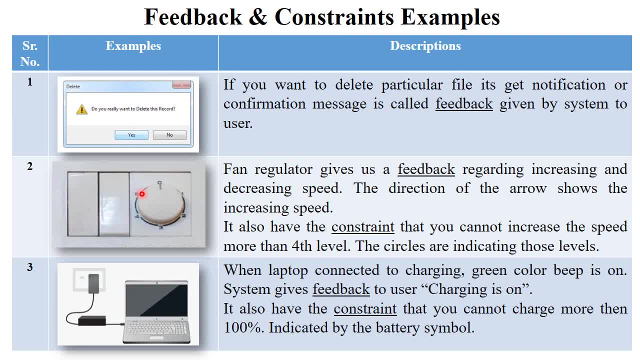 as constraint. This is called as limitations, right? So this is a feedback and constraints of fan regulator. Now the next one is laptop. When you connect your laptop for charging, at that time green color beep is on right- Means system gives a feedback that your charging. 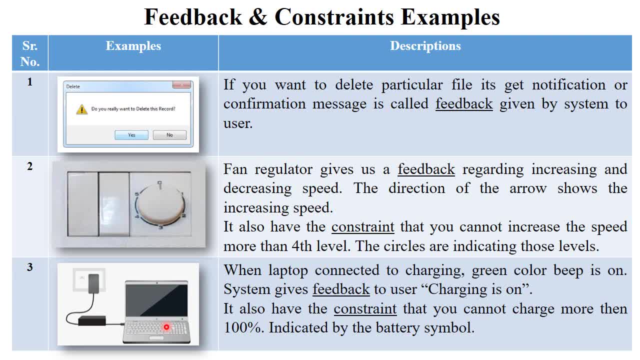 is on, right? So this is called as communication between system and the user, and the constraint is you cannot charge more than 100%, right? There is a particular battery symbol at the bottom of the corner, So this battery symbol indicate your battery percentage. So 100%. 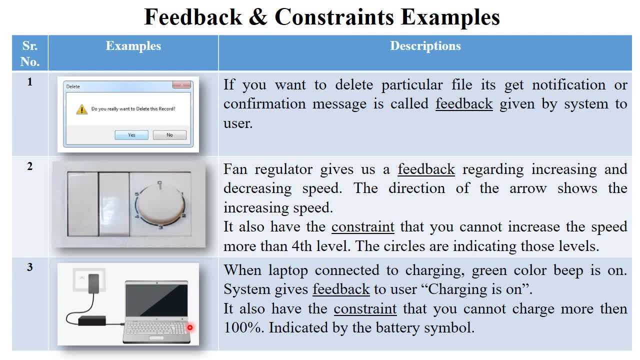 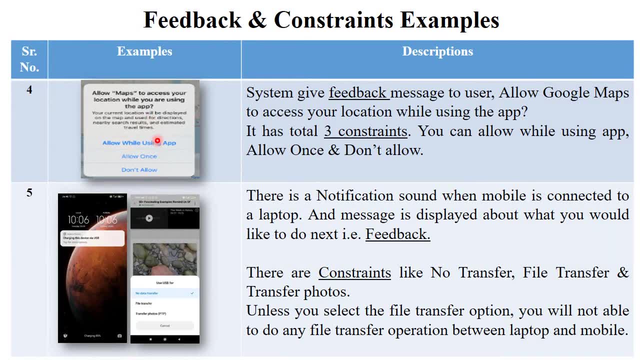 is a maximum. There is a limitations right. 100% means full, So this is called as feedback and constraint of laptop. Next, Now, next. I think you all are familiar with the Google Maps, right? So when you open a Google Map first time, right? So at that time they give. 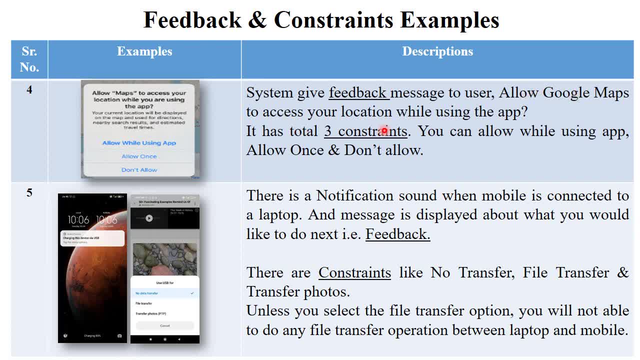 you a message like: allow Google Maps to access your location while using the app. This kind of message will be given right. So this is called as feedback. But there are total three options or three constraints. If you want to share the location, there are total. 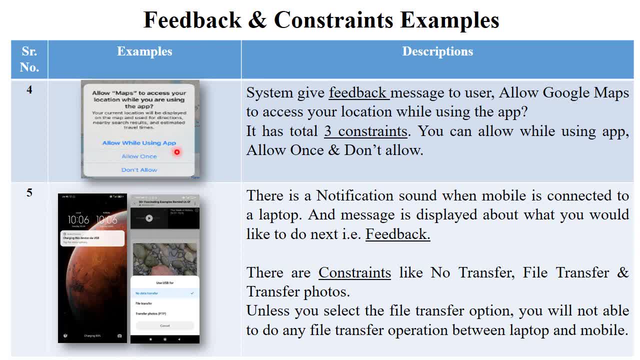 three constraints having there, Allow a location sharing while using the app. allow once or don't allow, right? So these three are called as constraints and this message is called as feedback and you need to follow a particular rules as per your requirement, right? 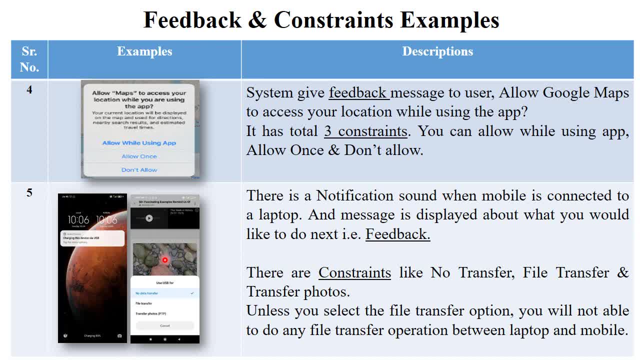 Now next. the next example is see here. When you connect your mobile to the laptop, at that time a particular notification sound is generated in your mobile right. There will be a particular notification sound. For example, you have a particular message that is displayed like this: So here there. 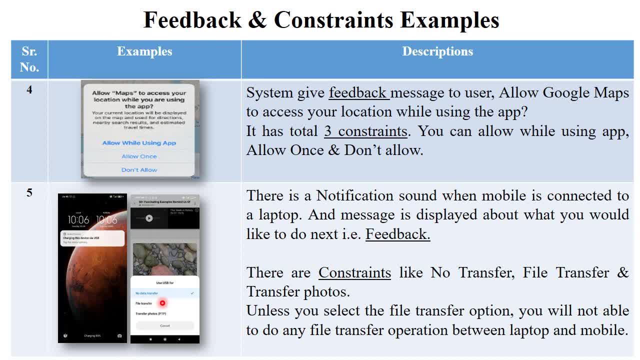 are all three constraints. you need to transfer a file transfer, transfer photos or no data transfer. So these three constraints are there. you need to apply or you need to choose any one constraint from this. There is no any fourth option. is there right Suppose? 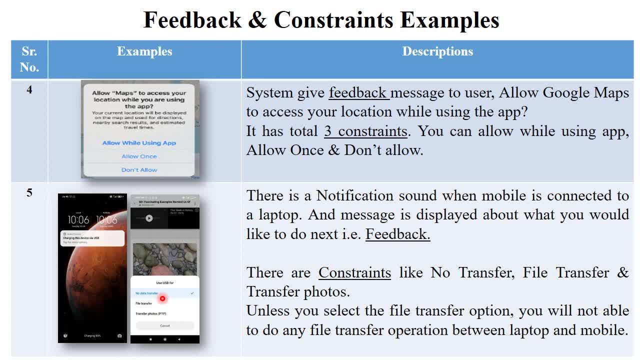 there is no. data transfer means just your mobile have charged as your laptop. file transfer means only file transfer and transfer Like this. there are no 4th option, is there right? So all these four curves left will be removed. True, Okay, But I do notice that we do need. 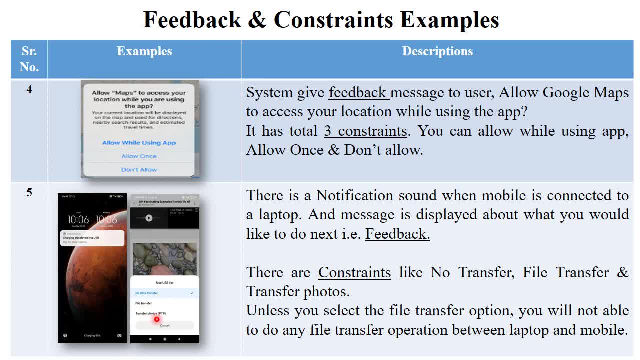 to include the checker as it is the Object指 scriptures, so I can put the enter as an middle to transfer the photos from mobile to laptop or laptop to mobile, right, so these three constraints have there and this is called as feedback message. complete message is called as feedback message.